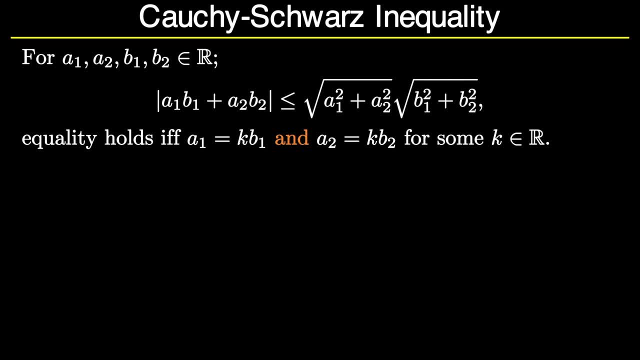 square root of a1 square plus a2 square into square root of b1 square plus b2 square, And the equality holds if, and only if, a1 is equal to kb1 and a2 is equal to kb2 for some real number, k. In other words, the equality holds if, and only if, the ratio of 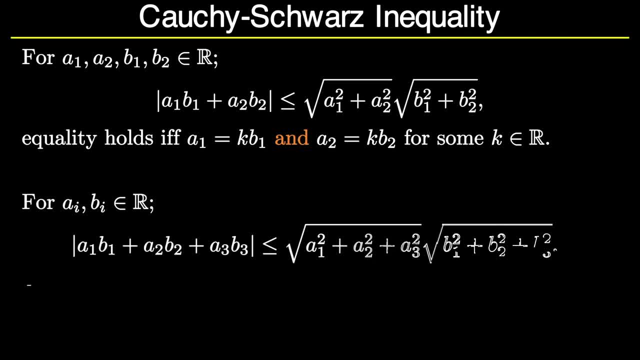 a1 and b1 is same as of a2 and b2.. Similarly, for three pairs of real numbers, we have this result. If you are learning CS Inequality first time, I recommend you to take your notebook out and write this inequality yourself. You will understand it better and quickly. 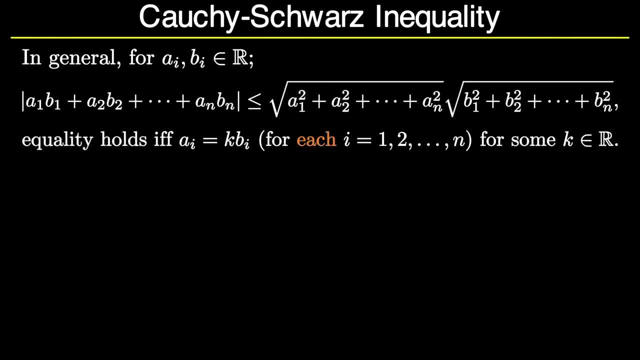 Don't stare the screen. The general statement of CS Inequality for n pairs of numbers is modulus of a1, b1 plus a2, b2 up to a, n, b, n is less than or equal to. is less than or equal to square root of a1 square plus a2. square up to a, n square into square root of b1.. 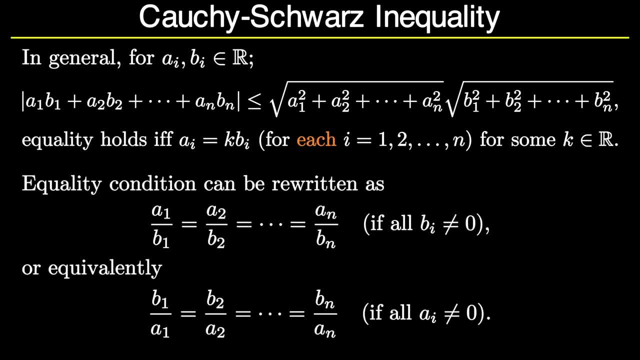 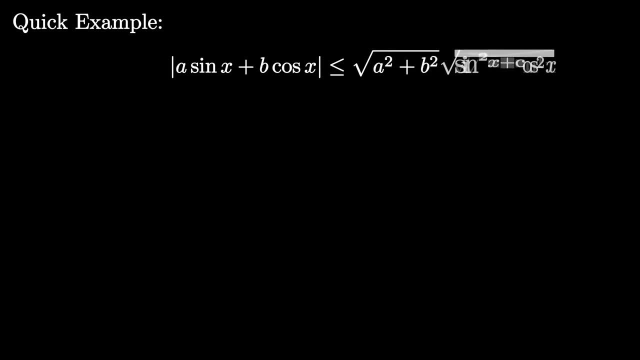 square into square root of b1 square plus b2 square up to bn square, And the equality holds if, and only if, a1 over b1 is equal to a2 over b2, up to an over bn. Let's see the strength of C-S inequality in this example. We immediately conclude that the maximum value 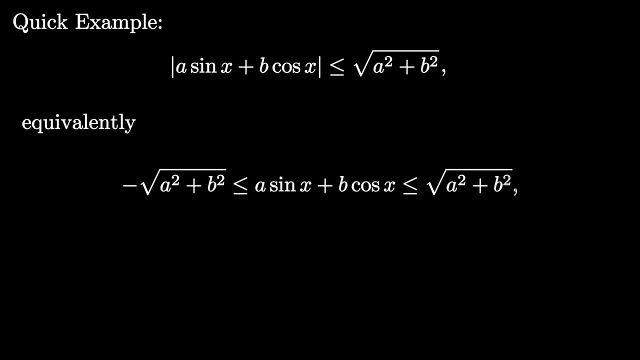 of modulus of a. sin x plus b. cos x is square root of a square plus b square. Many of you might have read the proof of this result in trigonometry as well. Notice that the C-S inequality proved this result instantly. Feel the strength of C-S inequality, But strength 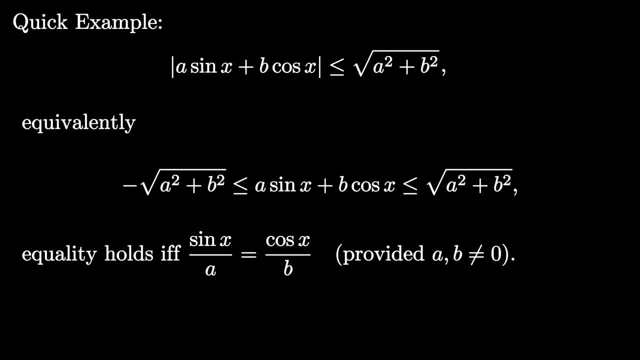 always comes at the cost. The hardware we put in proving the C-S inequality is the actual cost of this instant proof. I would like to digress for a moment and want to explore this point further. It is the nature of mathematics that 0. 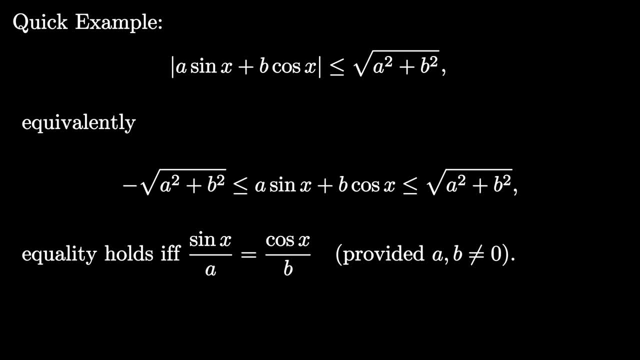 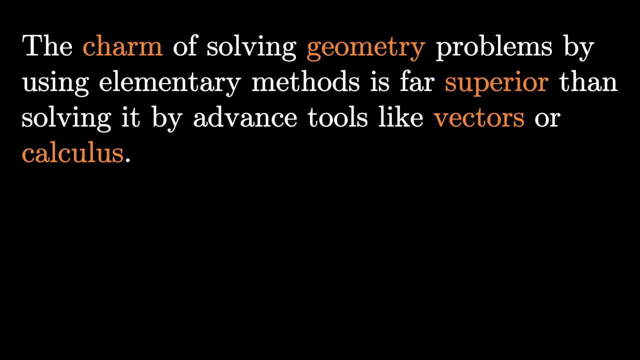 when we are equipped with stronger tools we are able to solve old problems in lesser time in comparison with elementary methods. But remember this does not diminish the importance of elementary methods. The charm of solving some geometry problem by using elementary methods is far superior than solving it by advanced tools like vectors or calculus. But 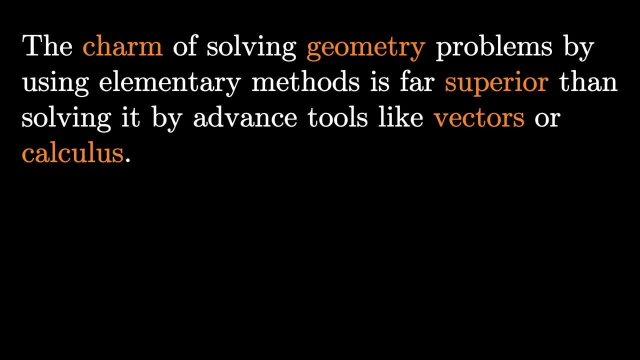 sometimes the elementary methods are so cumbersome or even incapable to solve some problems, then we have no choice other than advanced tools. In fact, such problems are the reasons we dig deeper and deeper and seek some breakthrough. that is how we invented calculus or linear algebra, for example. But in the perspective of problem solving you should explore many 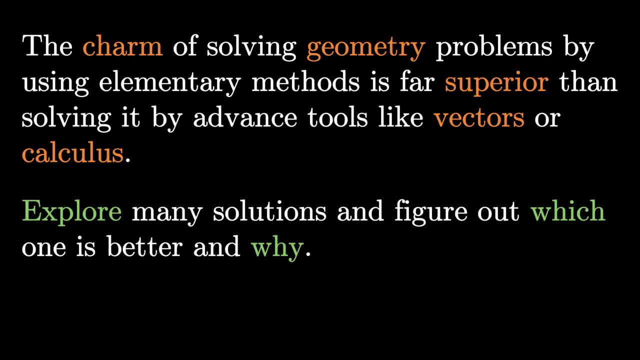 solutions and should ask yourself which method is better. Use the tools wisely, not blindly. I have personally seen many students who blindly use derivatives. when they get a problem on finding the range of some function, They think that the derivatives is the only tool to tackle. 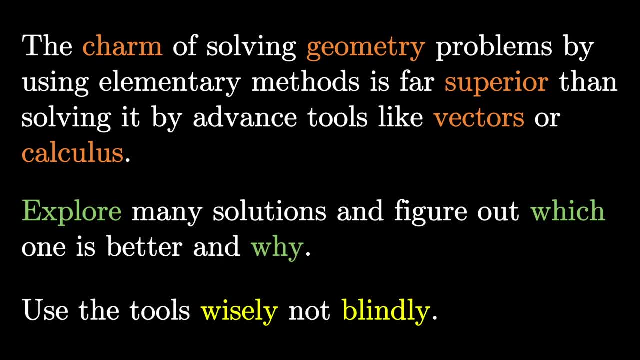 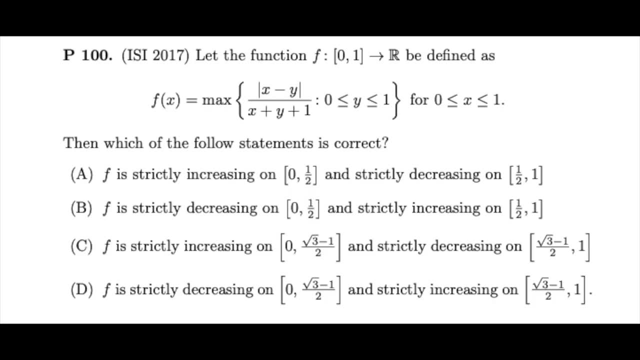 such problems. but it is not the truth. We can pose a problem whose solution based on calculus is complex, mechanical and dull in comparison to elementary methods. that can pup's us towards some unfamiliaruber합 methods which gives imaginative and beautiful solution. For example, try out this nice ISI. 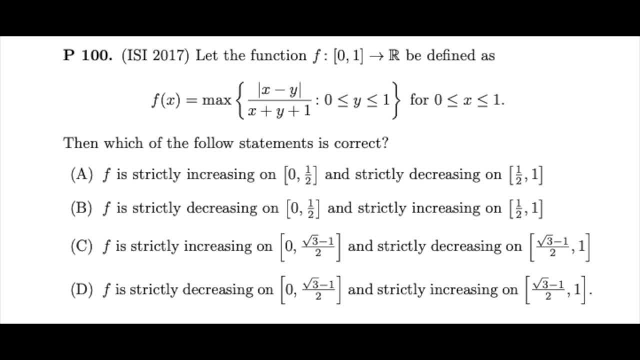 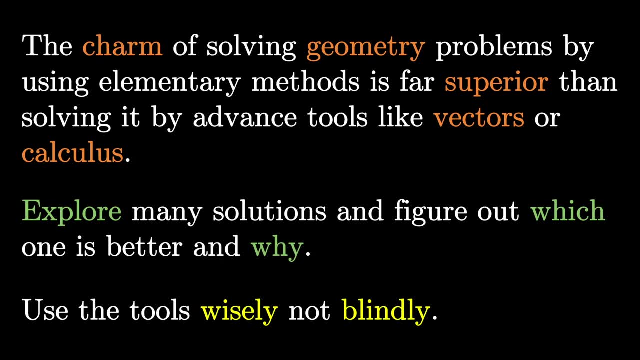 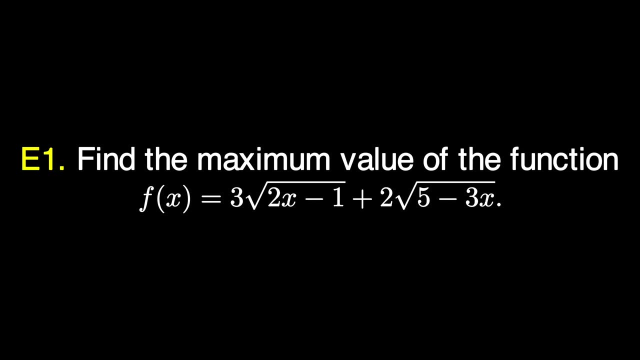 problem from my book Algebra, Volume 1.. So, finally, the crux of the whole discussion is what I just said before and I repeat: use the tools wisely, not blindly. Now let's come back to the CS inequality. Let's take the first example. What a coincidence. I was just advocating non-calculus solutions to find. 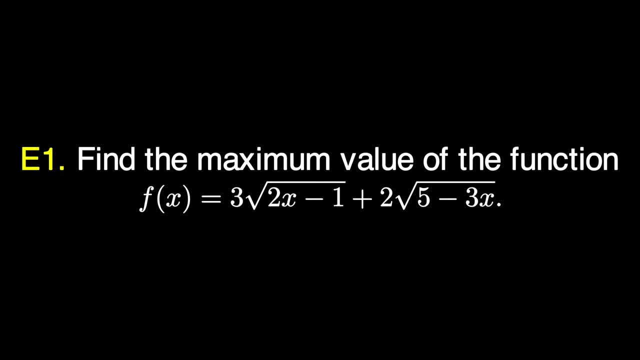 the range of some function and we get the problem on finding the maximum value of the function. fx is equal to 3 square root of 2x minus 1 plus twice square root of 5 minus 3x. Definitely we are not going to use calculus. I can assure that the derivative will make. 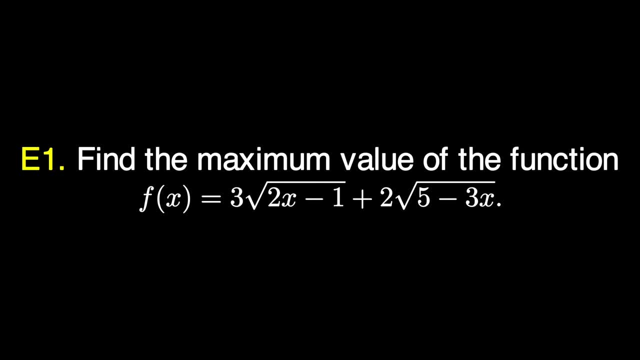 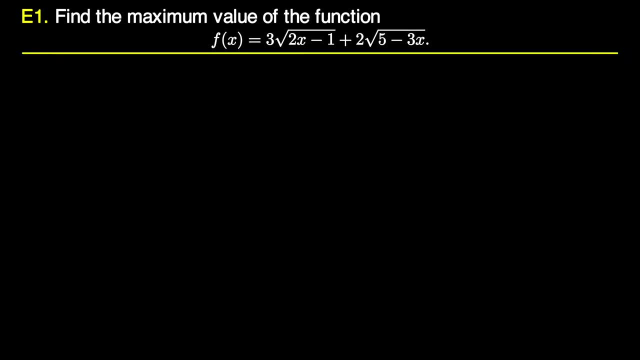 this problem agreeable, And I am sure, like me, you are a devotee of imaginative and beautiful work. Otherwise, there is no reason to stick with me so far. So we are going to use CS inequality. Let's see what we can do with CS inequality in this. 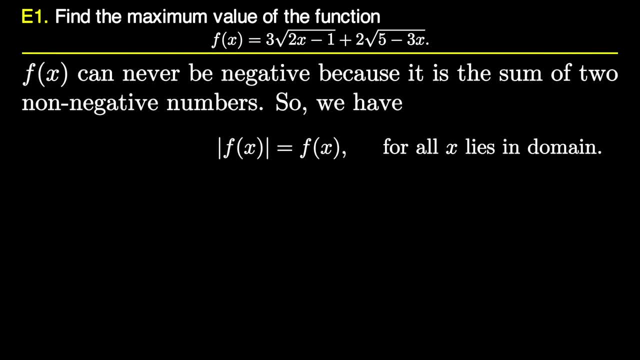 problem. We can quickly observe that fx can never be negative because it is the sum of two non-negative numbers. So modulus of fx is equal to fx, And now we can apply the CS inequality That gives fx is less than or equal to square root. 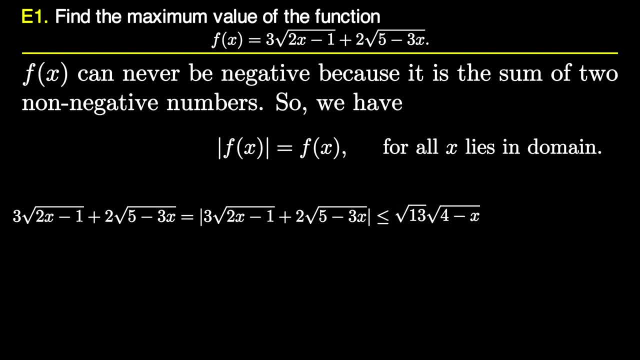 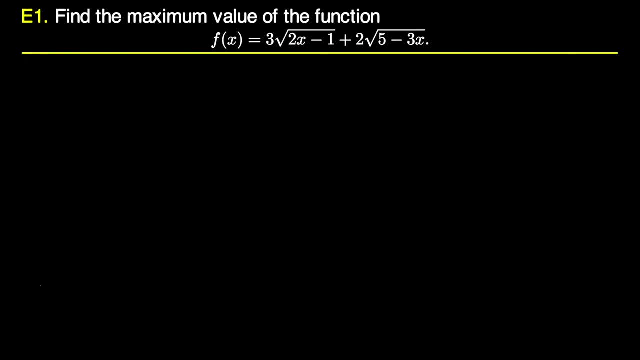 of 13 into square root of 4 minus x, But this is not a constant value. So what should we do now? Can we apply CS inequality cleverly that serves our purpose? The answer is yes. Our goal is to make the RHS a constant, So we manipulate fx to be. 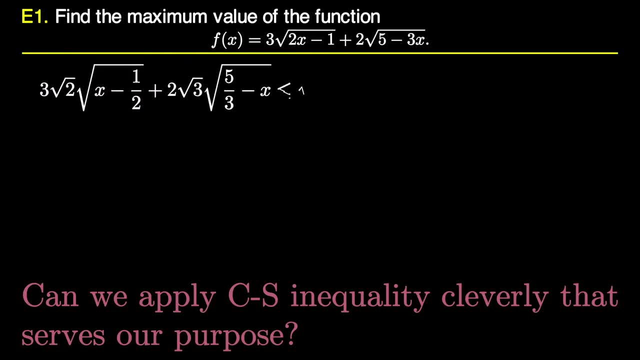 fx in this way, And then we apply CS inequality. This time we are getting the RHS constant. We are getting fx is less than or equal to square root of 35. Can we conclude that the maximum value of fx is square root of 35?? The answer is not. now. 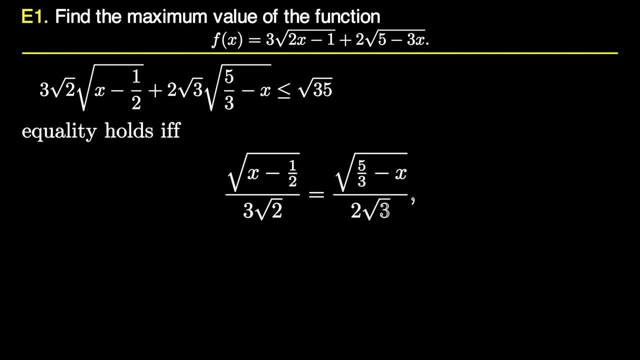 We have to actually show that there exists some x for which the equality holds, And the equality holds if, and only if, these two ratios are equal. That gives, x is equal to 6 over 5.. But there is one more pitfall we have to fix. We have to check whether 6 over 5 lies in. 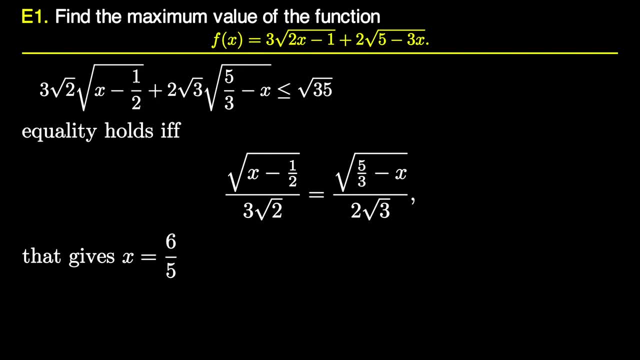 the domain of fx or not. So the question is: what is the domain of fx? It is easy to find. that is the interval from half to 5 over 3.. And we are lucky that 6 over 5 lies in the interval. Now we can safely 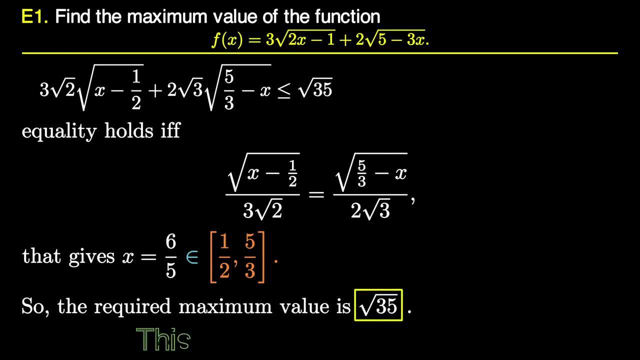 say that square root of 35 is the maximum value of fx, And this completes the solution. If the video is helpful for you, then why are you hesitating to hit the like button? Hit it now. Making such amazing videos requires a lot of efforts. Your one token of appreciation. 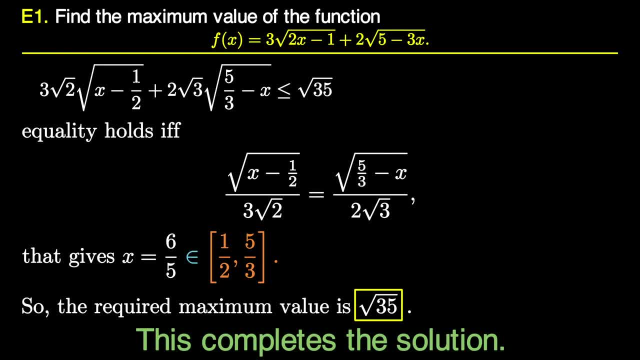 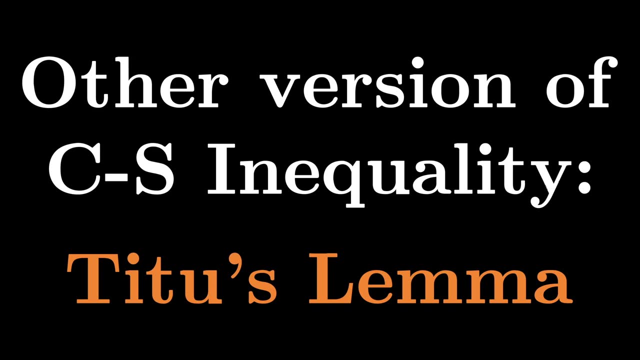 motivates me to produce more videos like this. Thank you, So be vocal to give your opinion in the comment section, Because it matters a lot. Let's move on. We have another version of CSA inequality that is popularly known as T2's lemma In. 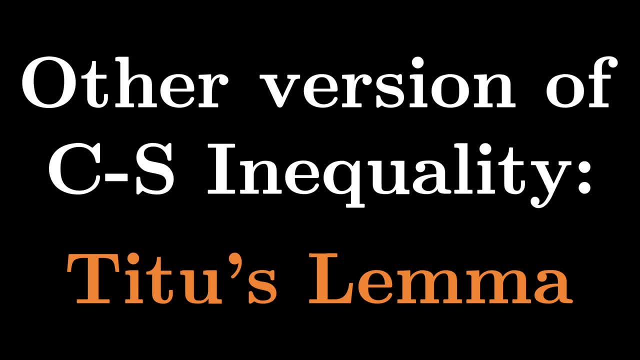 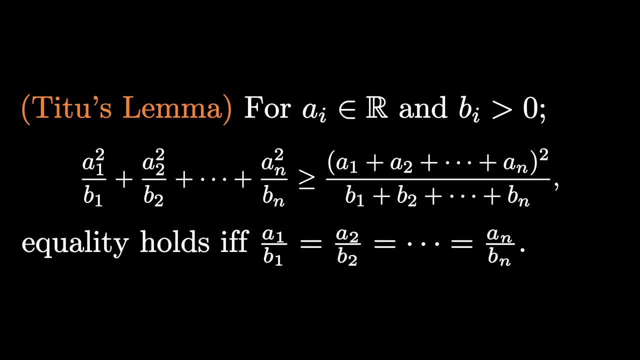 fact this version is more popular than the original one because it is used frequently. This is the general version of T2's lemma. I repeat: if you are learning it first time, make sure you write it yourself. Notice that the difference that in the previous version both ai's and bi's can be any real number. 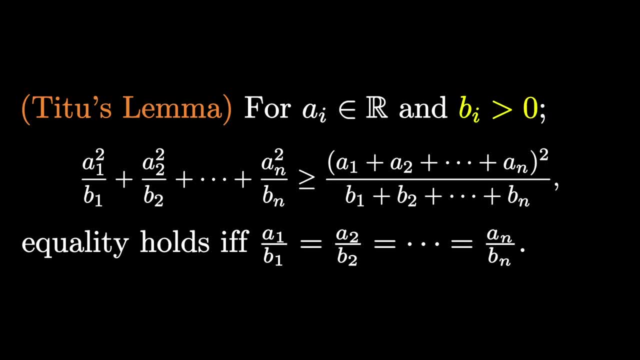 But in T2's lemma bi's are positive. Let me read out the statement for you. For real ai's and positive bi's we have a1 square over b1 plus a2 square over b2 up to an square of bn is greater than or equal to a1 plus a2 up to an whole square upon b1 plus b2 up. 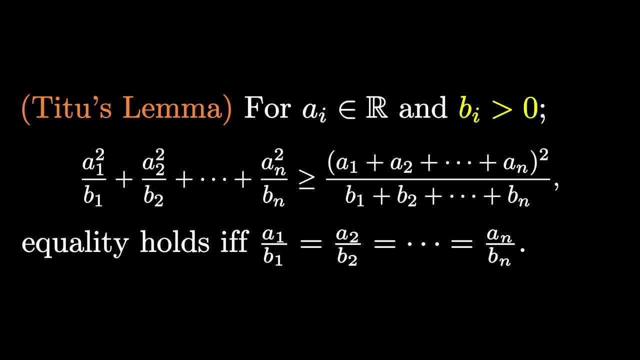 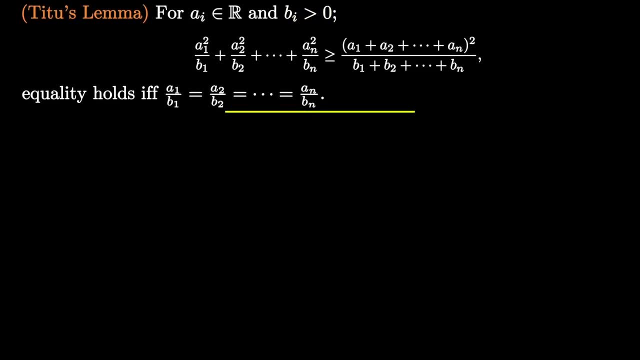 to bn, And the equality holds if, and only if, a1 over b1 is equal to a2 over b2, up to an over bn. We can prove it by writing modulus of a1 plus a2 up to an in this way and then: 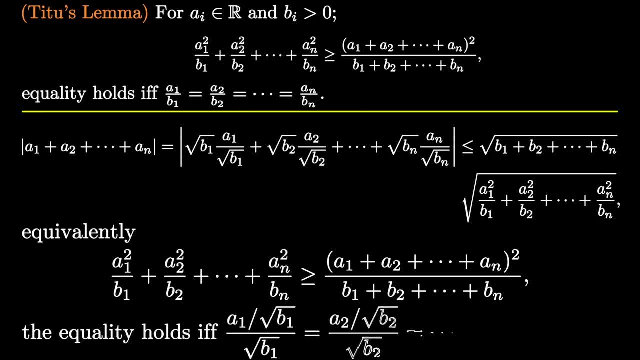 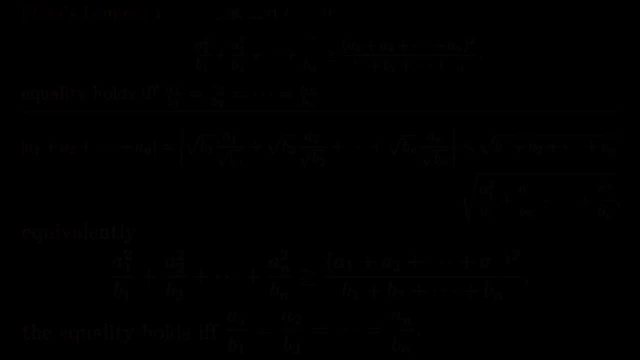 applying the CSA inequality And we get what we wanted. That's it. Hopefully, now you are convinced that T2's lemma is nothing but another version of CSA inequality, Let's try out a problem to demonstrate the use of T2's Lemma. Let a, b and c be positive. 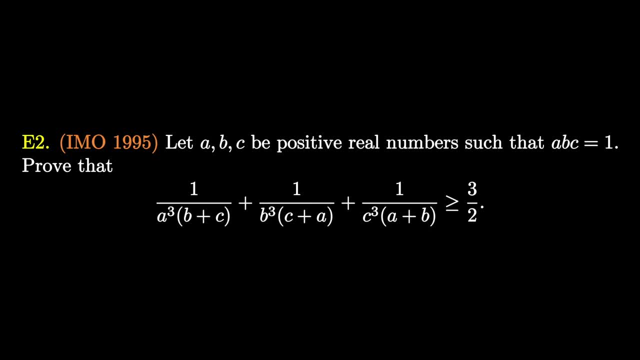 real number, such that abc is equal to 1.. Prove that 1 over a cube into b plus c plus 1 over b cube into c plus a plus 1 over c cube into a plus b is greater than or equal to 3 over. 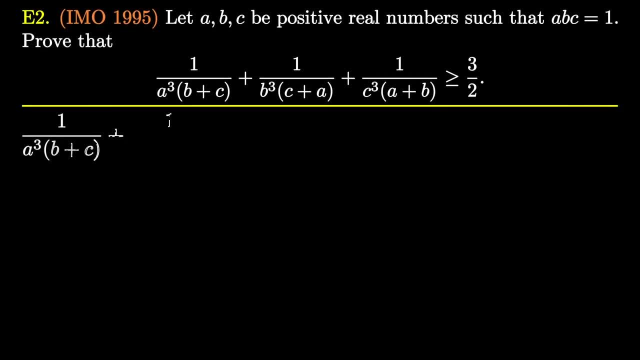 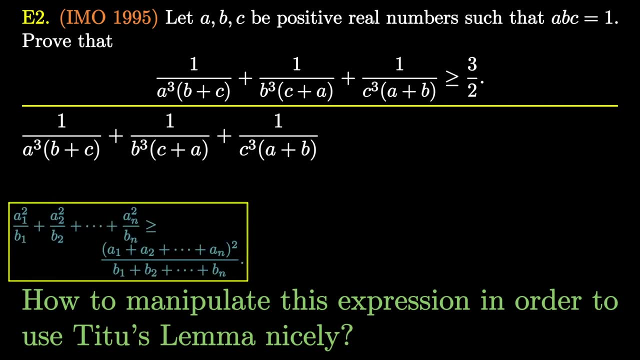 2. Ask yourself how to manipulate this expression in order to use T2's lemma. nicely, Recall the statement of T2's lemma and think: If you want, you can pause the video. We can write it in this way. Now we apply T2's lemma and we get this inequality. 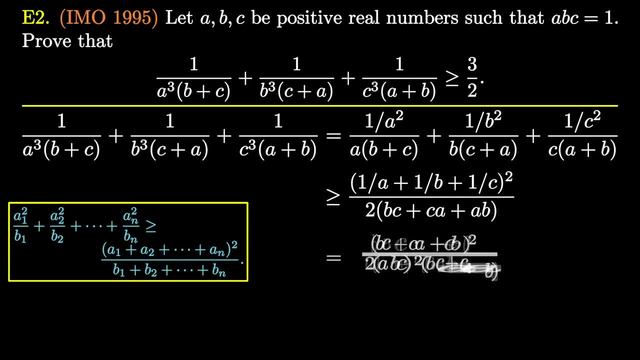 Now we have the sum of three ratios is greater than or equal to BC plus CA plus AB upon 2.. Now what? What should we do next? Can we find the value of BC plus CA plus AB? The answer is no. We are given only the value of ABC and from that they are infinite possible.